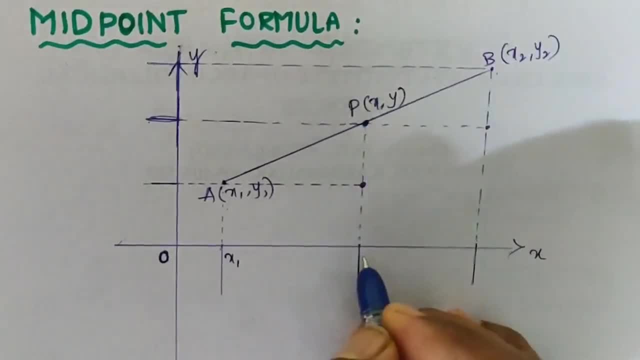 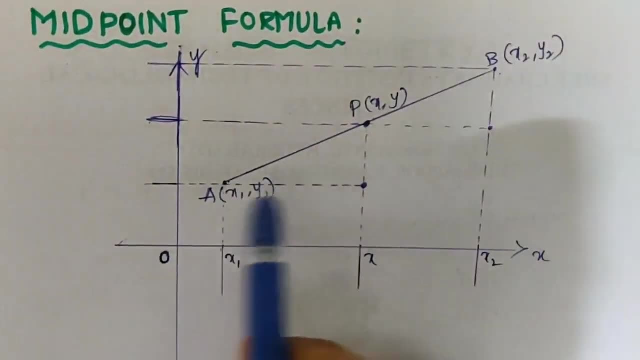 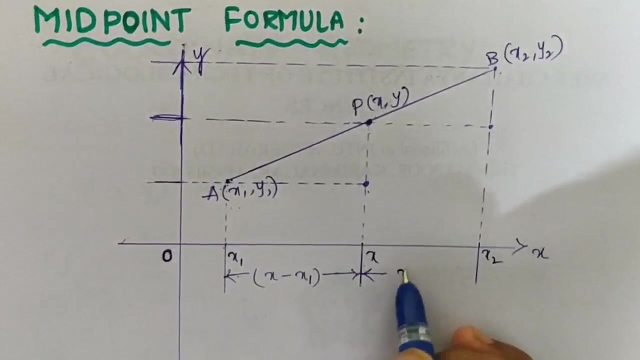 And here the x coordinate is x and here the x coordinate is x2.. The distance between these two points on x axis is x minus x1.. So it will be x minus x1, and here the distance is x2 minus x. We need to write all these. 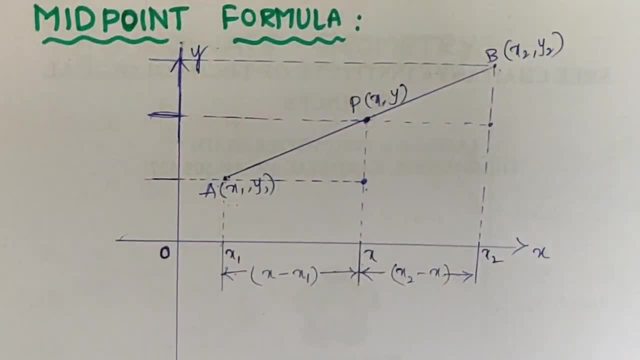 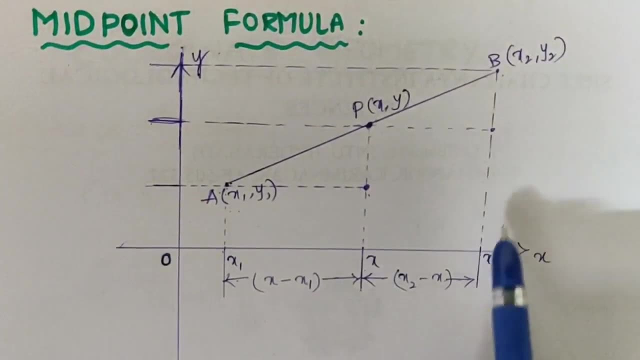 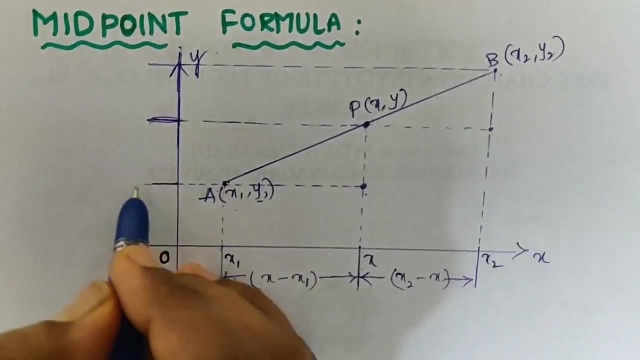 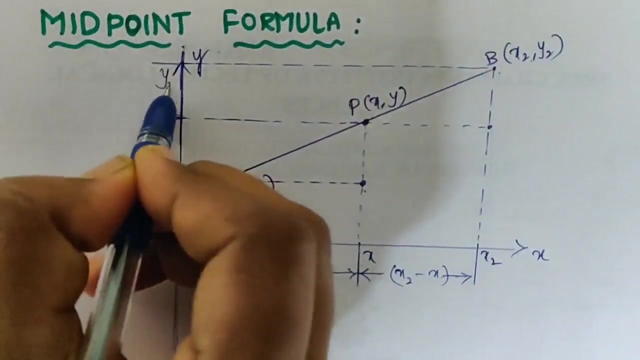 Measurements of all the points from x axis and y axis to find out the midpoint. And the same thing: here, the distance from point A to y axis is y1.. We need to take the y coordinate: Here it is y1 and here it is y and here it is y2.. 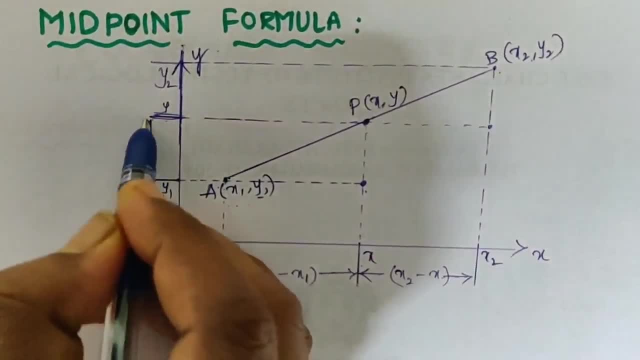 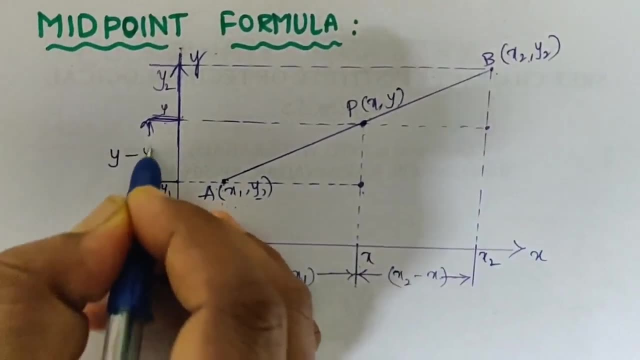 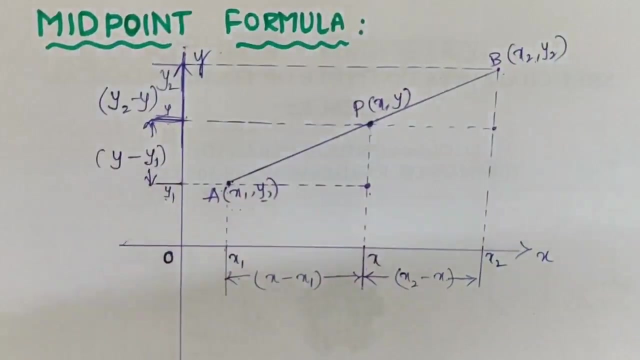 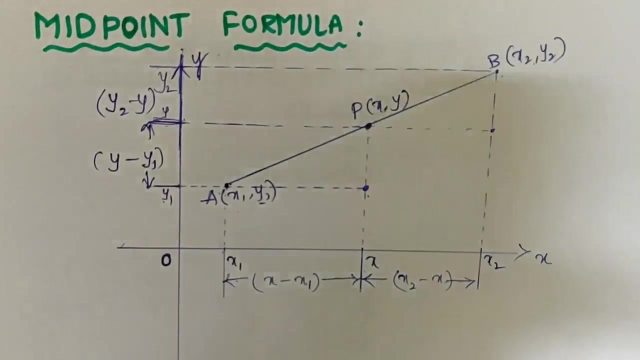 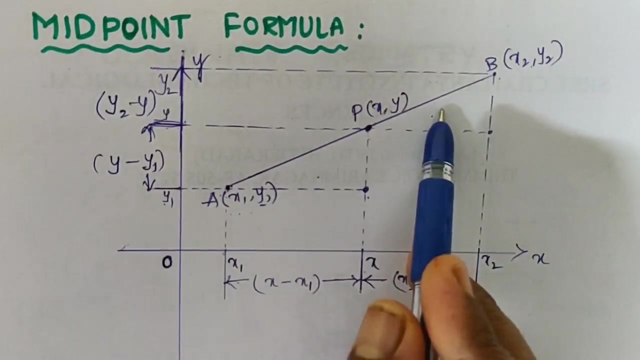 Now the distance between these two points will become The difference between the y coordinates, right, So that will be y minus y1.. Here it is y2 minus y, and we got all the distances on x axis and y axis. Now we have to find this midpoint. for that purpose, I am taking these two as the similar triangles. ok, 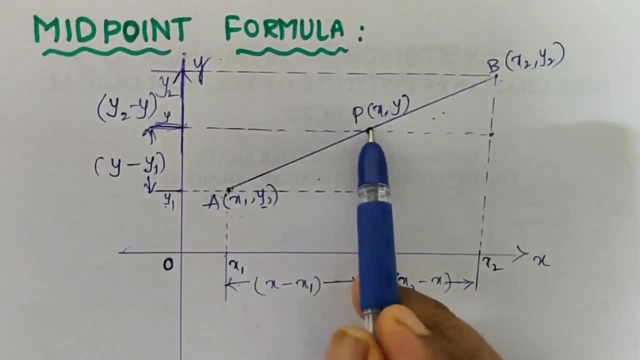 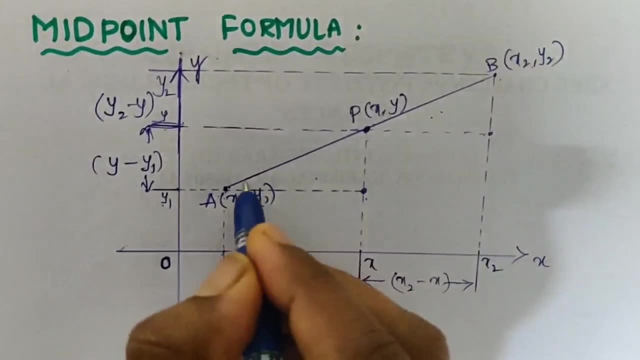 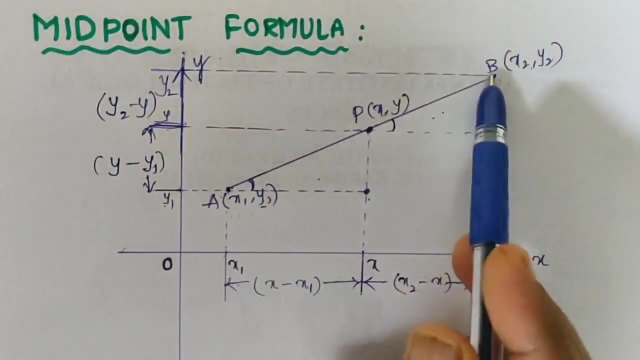 Similar and equivalent. Why? because it is a midpoint and these two are the parallel lines, So the angle here and the angle at P will be equal, Because the same line having the inclination with the parallel lines, So the two angles will be equal. 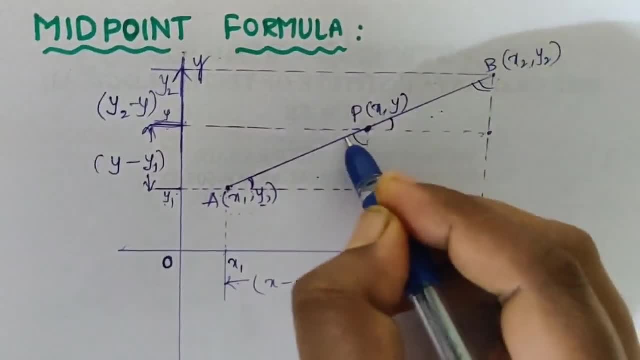 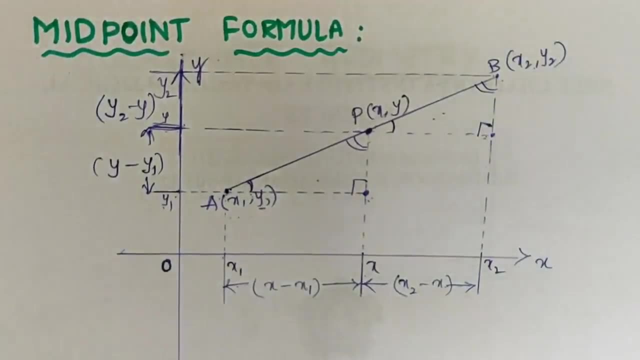 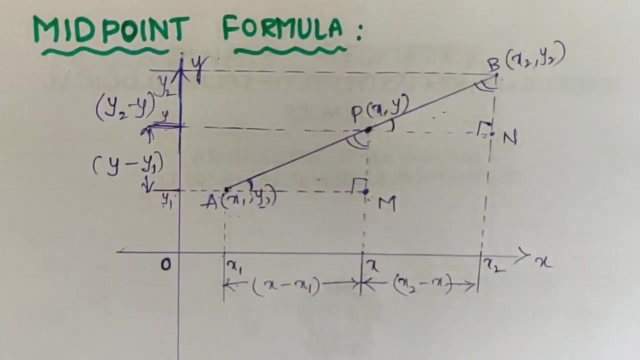 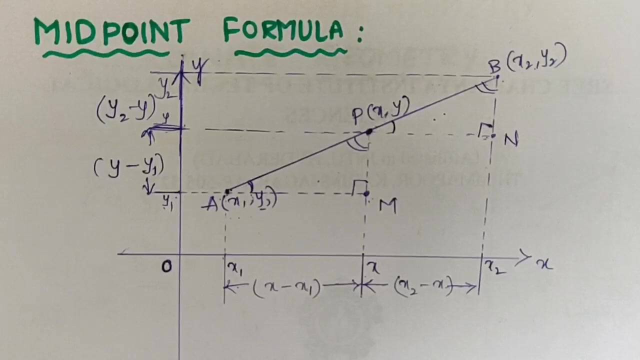 And here also same. these two angles will be equal right, And obviously we know it is a Perpendicular angle. Now I am naming it as M and it as N. Ok, the construction is completed. Now from this we need to find the P value, that is, x, comma, y values. 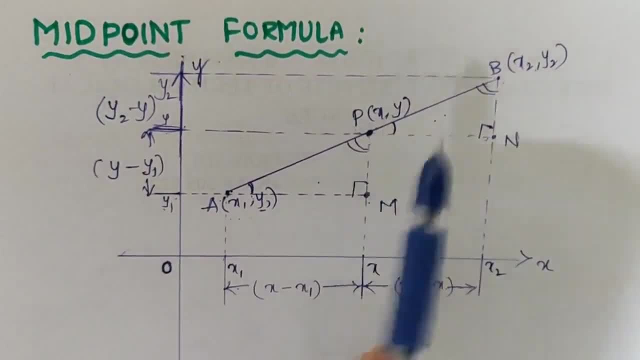 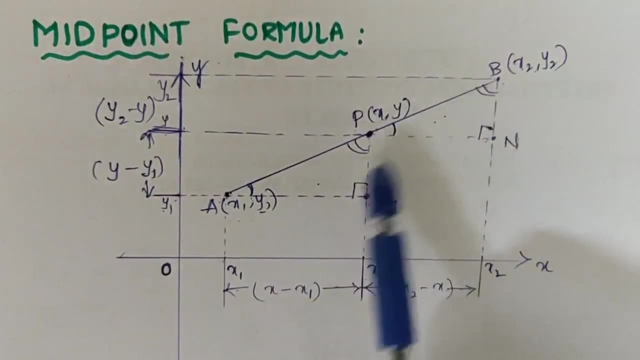 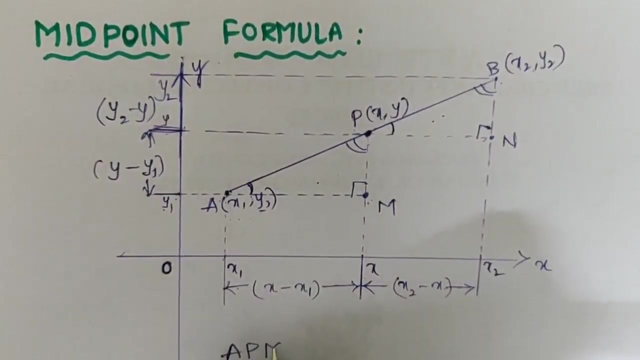 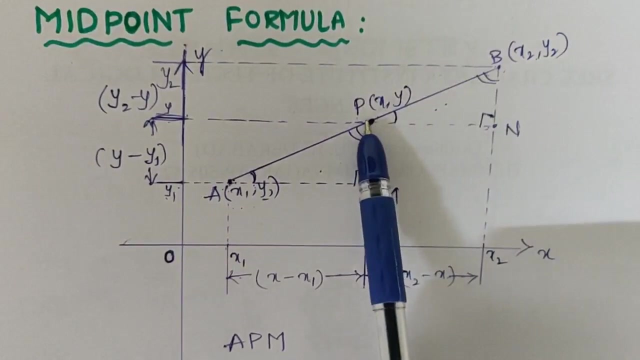 So now we have to find this P value, The coordinates of P. we need to find What are the coordinates of P, x and y. For that purpose, I am taking these two, The help of these two triangles. what are those here? the triangle APM: ok, triangle APM, which is similar to P, B, N, right. 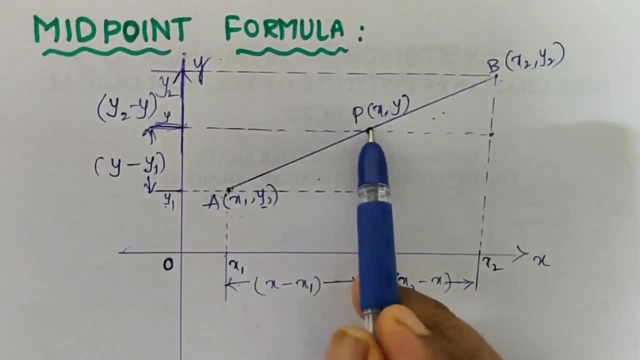 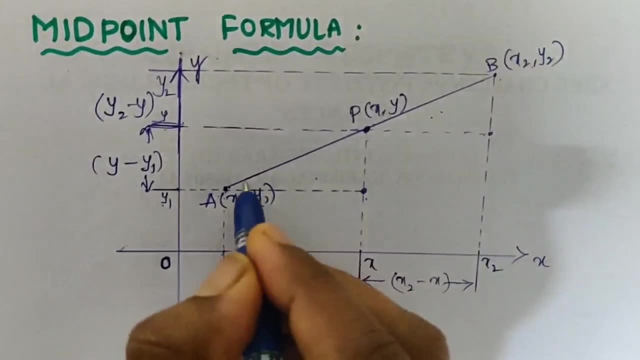 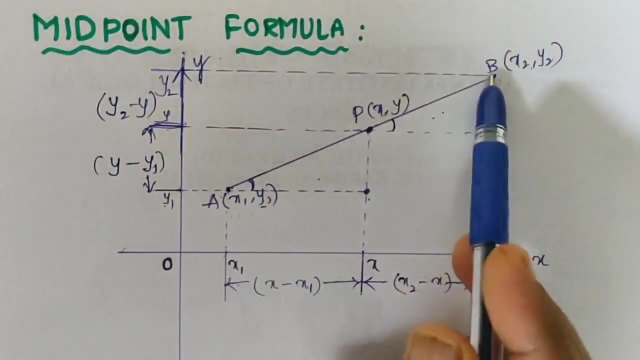 Similar and equivalent. Why? because it is a midpoint and these two are the parallel lines, So the angle here and the angle at P will be equal, Because the same line having the inclination with the parallel lines, So the two angles will be equal. 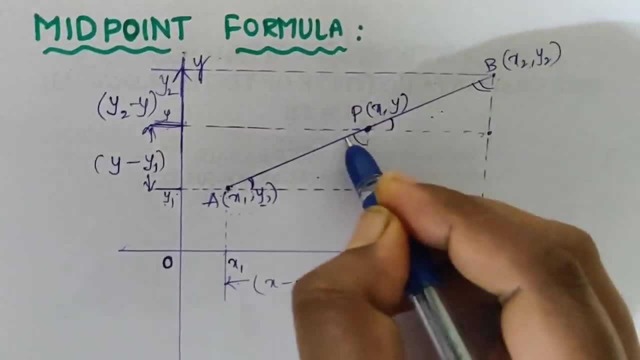 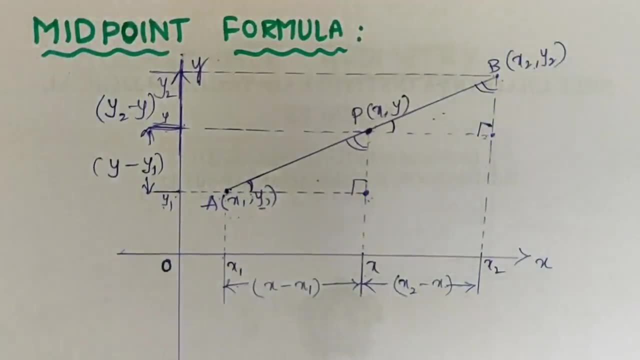 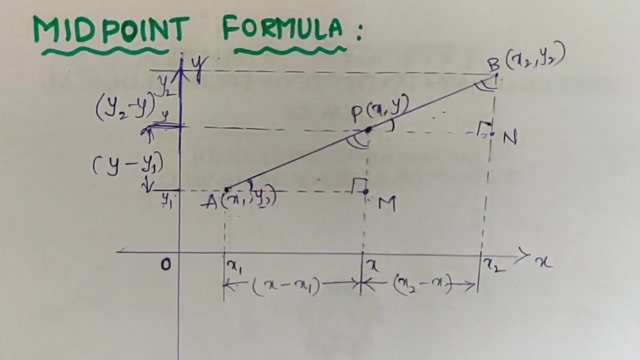 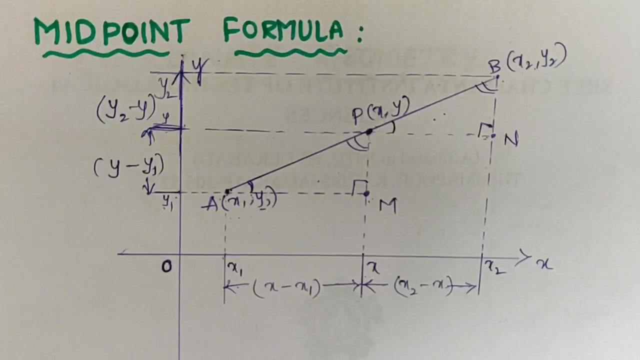 And here also same. these two angles will be equal right, And obviously we know it is a Perpendicular angle. now I am naming it as M and it as N. ok, the construction is completed. now from this we need to find the P value, that is, x, comma, y values. so now we have to find this P value, the coordinates of P. we need to find what are the coordinates of P, x and y. 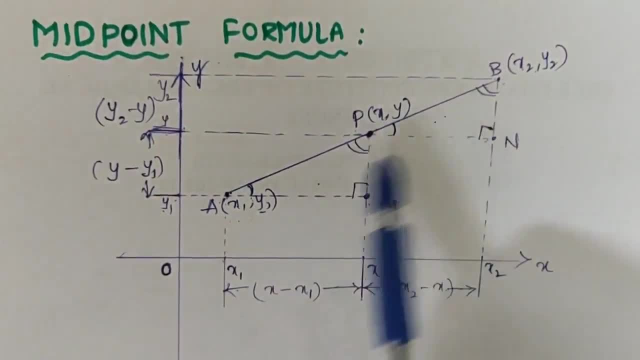 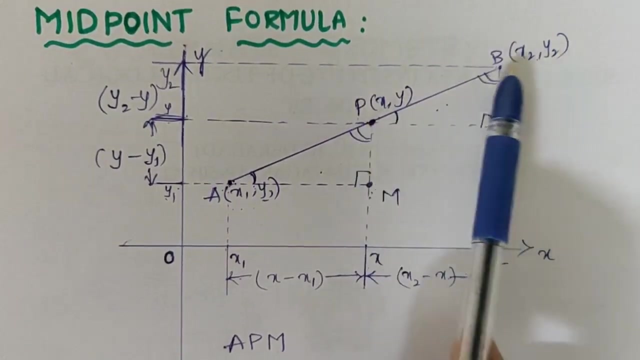 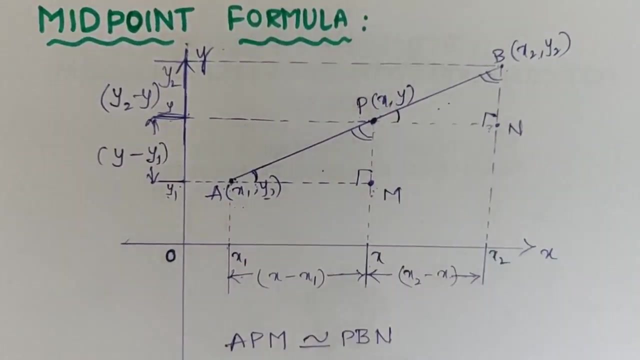 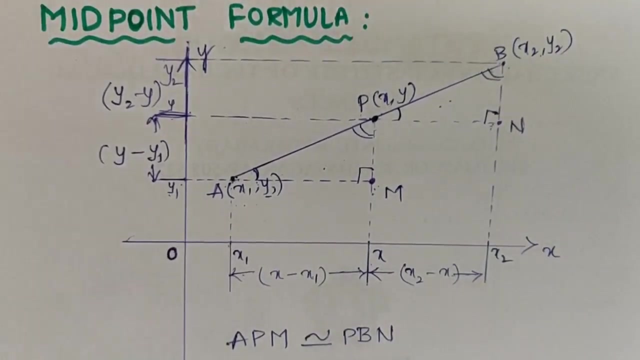 For that purpose, I am taking these two, The help of these two triangles. what are those here? the triangle APM. ok, triangle APM, which is similar to P B N, right, so it is similar to P B N. so now, by comparing these two triangles, we need to find the x value and y value. 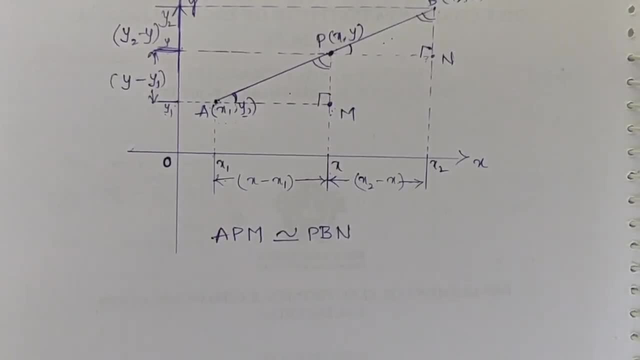 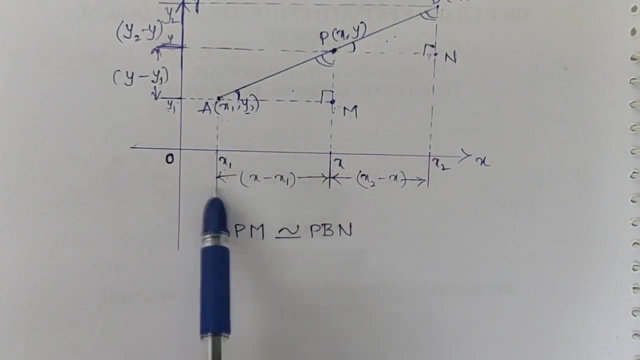 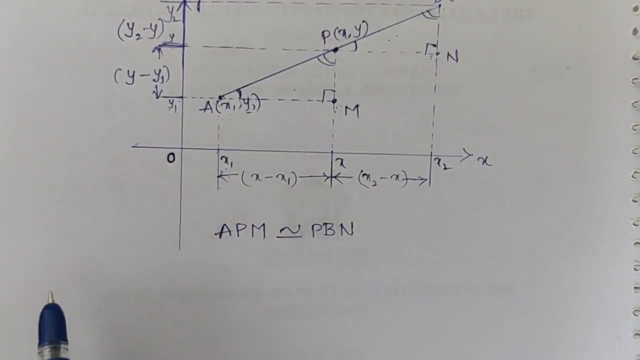 So from These two triangles I am comparing AM with P, N. ok, the first comparison because we need X coordinate as well as Y coordinates. so I am comparing with one X coordinate and one Y coordinate. so I am writing that. So what we can write here, 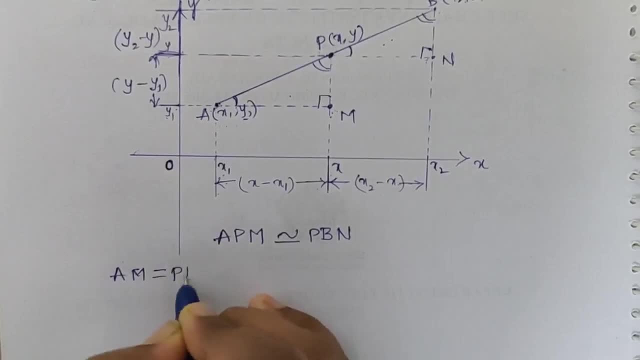 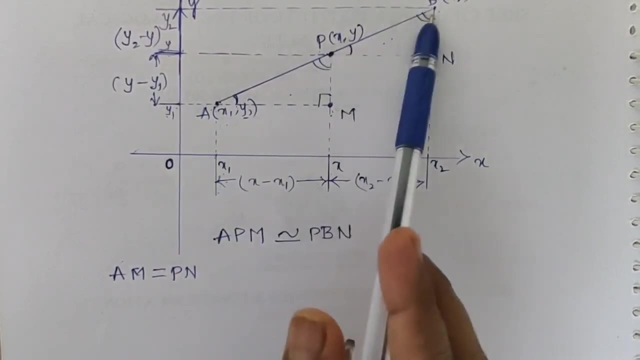 AM equals to PN, because these two are the similar time triangles, so The base is equal, it's O equal to this base and this hypotenuse equal to this hypotenuse and Pm equals to Bn, always. So, by comparing these two, what you will get? what is the value of Am, which is same as this? 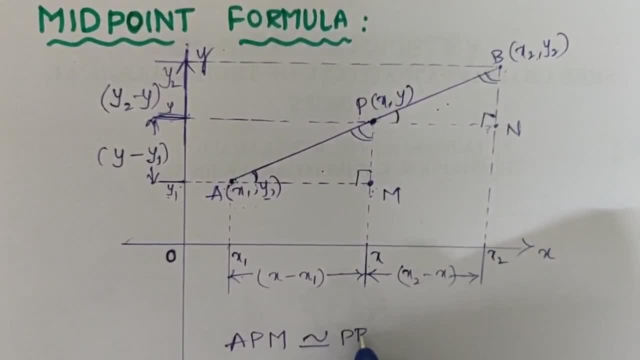 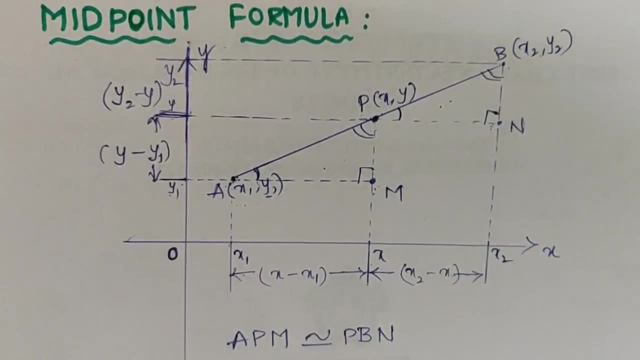 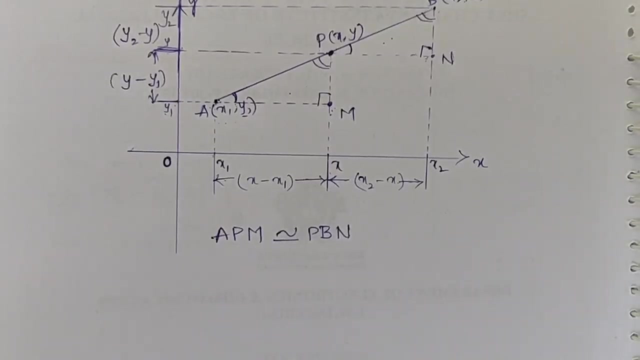 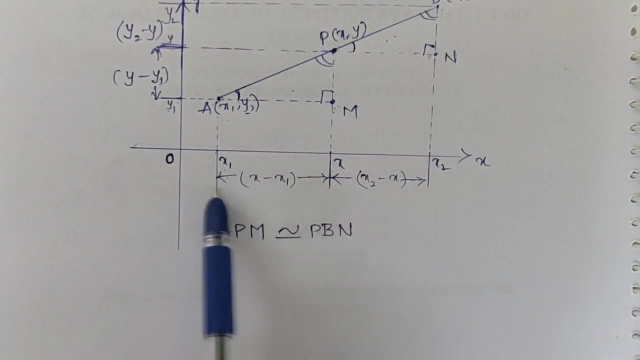 So it is similar to P B N. so now, by comparing these two triangles, we need to find the x value and y value. So from these two triangles, I am comparing AM with P N. Ok, the first comparison, because we need x coordinate as well as y coordinate. so I am comparing with one x coordinate and one y coordinate. 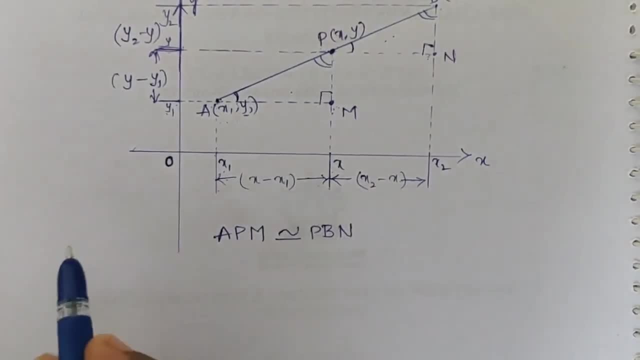 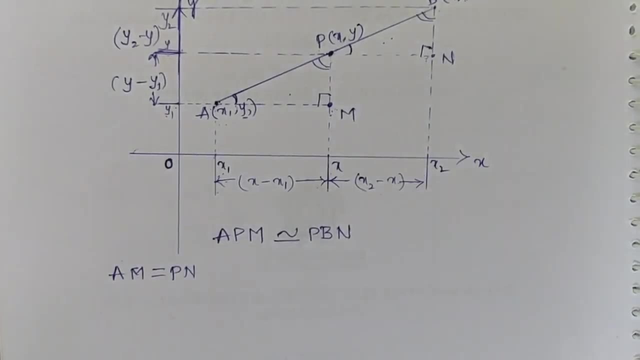 So I am writing that. So what we can write here: A M Equals to P N, because these two are the similar triangles. So The base is equal to equal to this base, and this hypotenuse equal to this hypotenuse, and Pm equals to Bn, always. 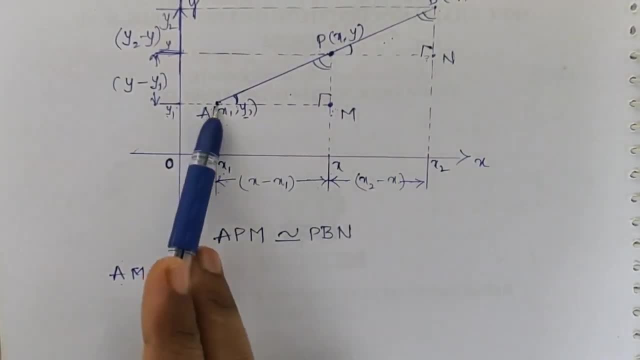 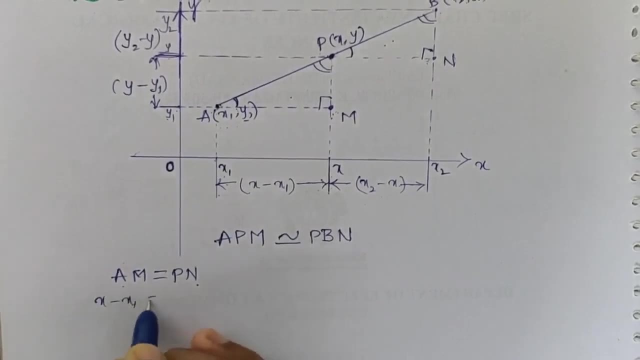 So by comparing these two, what you will get? what is the value of Am, which is same as this one? right, that is x minus x1. equals to what is Pn here, x2 minus x. So by solving this, what you will get, taking the x terms, one side, that is x plus x. when you take this x2 left. 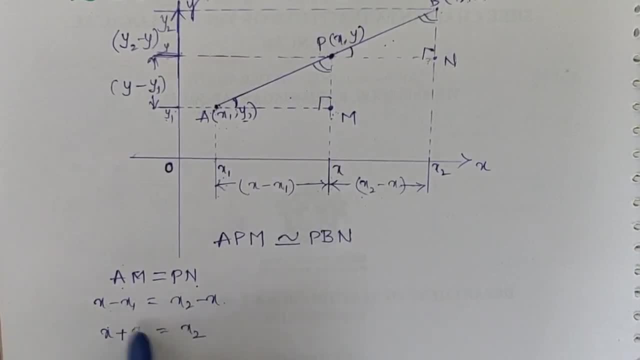 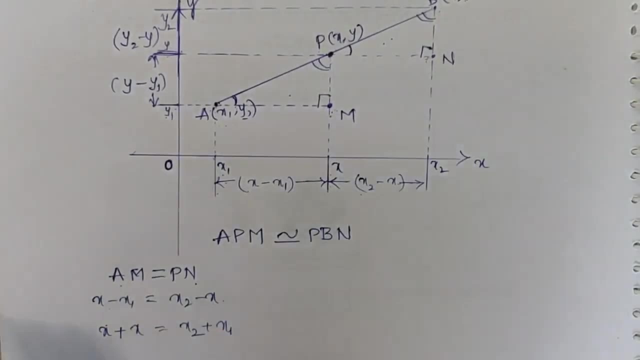 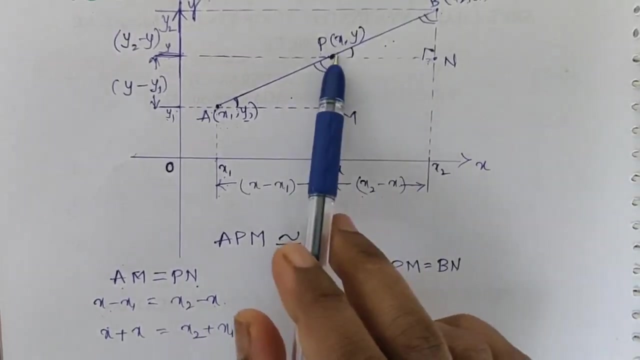 side. it will get plus x and x2 here, and this x1 will be plus x1. ok. In a similar way for the y coordinate, I am comparing Pm with Bn. ok, This Pm is equals to Bn, So I am comparing. 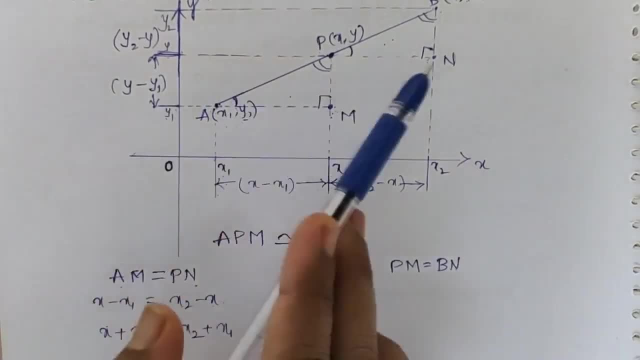 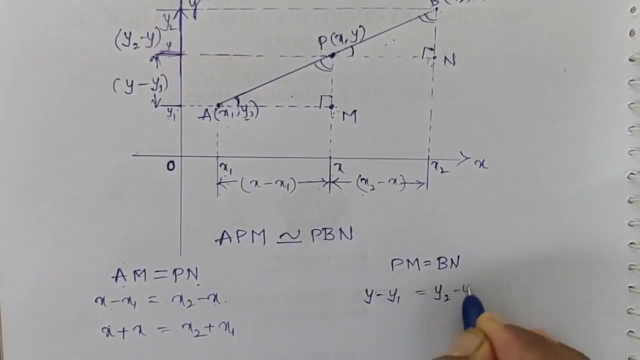 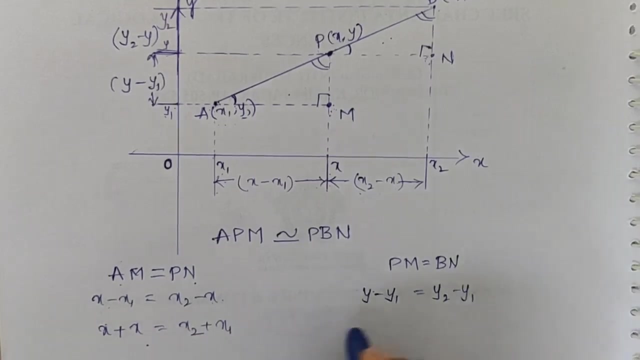 these two, we will get What is the Pm value here? y minus y1, which is equal to y2 minus y1. clear In the same way we need to solve, however we solve this one. you need to solve like this: So y plus. 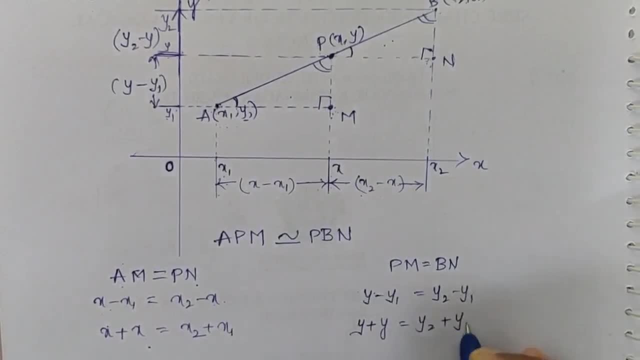 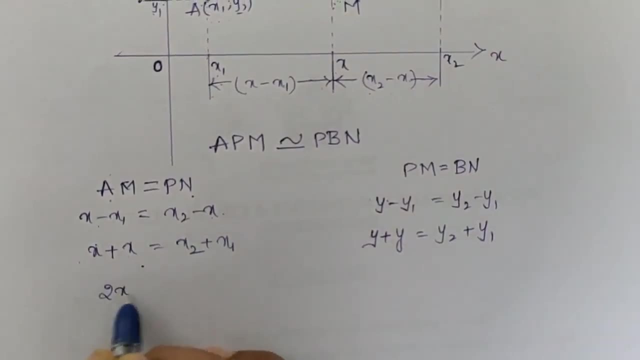 y equals to y2 plus y1. ok, After that here, x plus x is 2x equals to y2 plus y1. ok, So x1 plus x2 and x will become x1 plus x2. this will be upon 2. ok, This is a x coordinate. 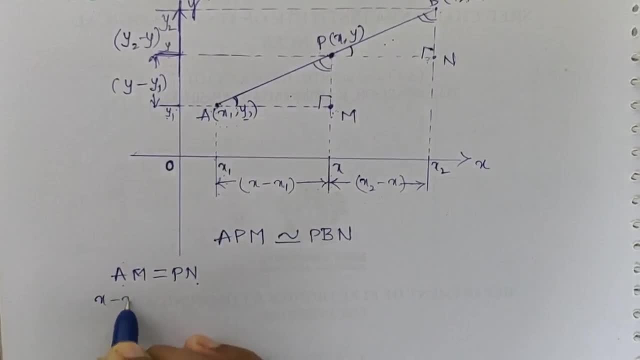 one right, that is x minus x1, equals to what is Pn here, x2 minus x. So by solving this, what you will get, taking the x terms one side, that is x plus x. when you take this x2 left side, it will get plus x and x2 here, and this x1 will be plus x1. ok, In a similar way for 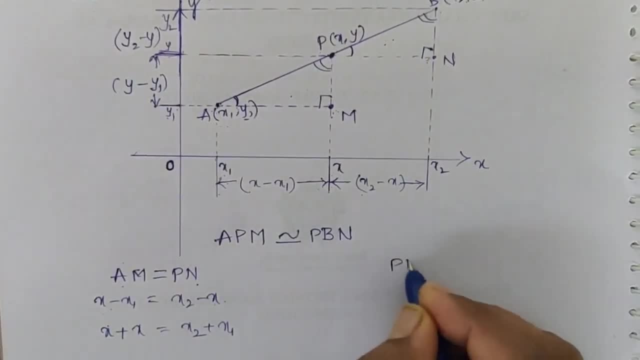 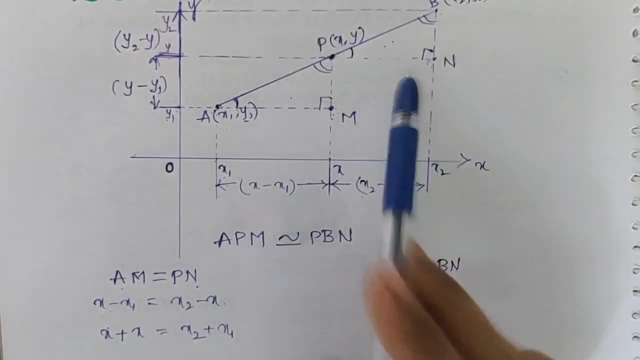 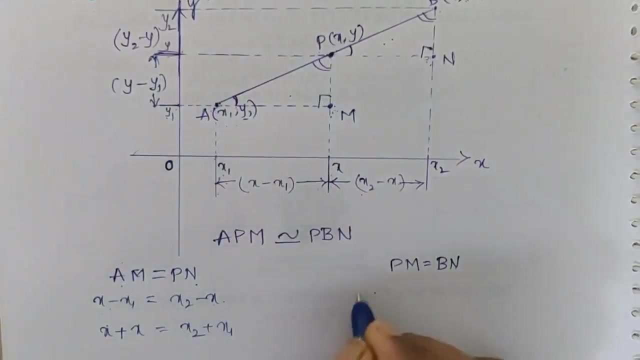 the y coordinate. I am comparing Pm with Bn. ok, This Pm is equals to Bn, So I am comparing these two. we will get What is the Pm value here: y minus y1, which is equal to y2 minus y1. clear In the same. 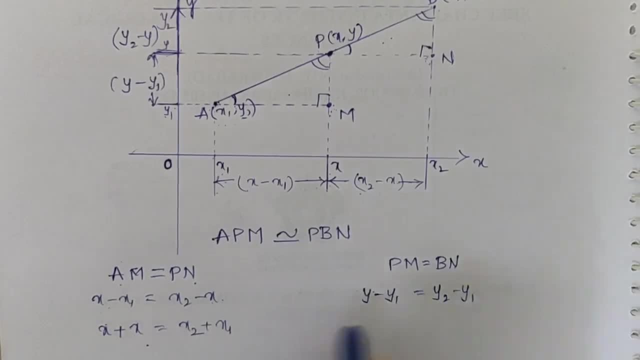 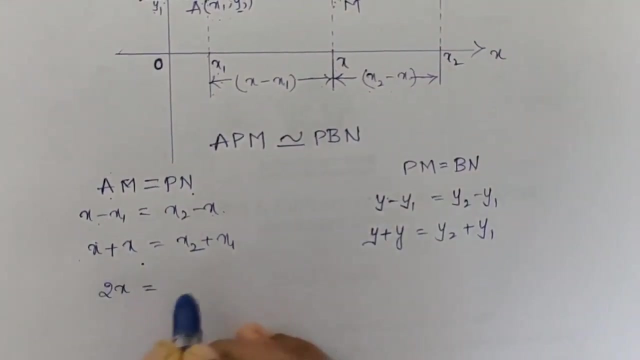 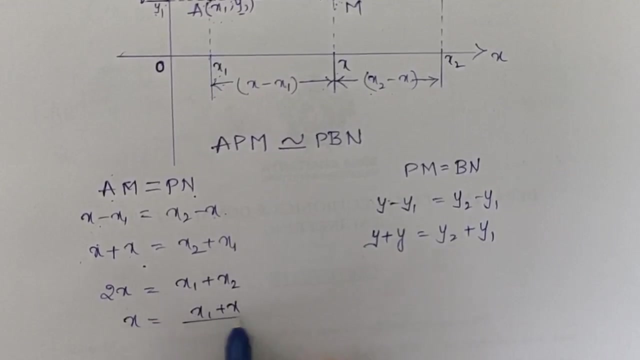 way we need to solve. however we solved this one. you need to solve like this: So y plus y equals to y2 plus y1. ok, After that, here, x plus x is 2x equals to y2 plus y1. right, x1 plus x2 and x will become x1 plus x2. this will be upon 2. ok, This is a x coordinate, and. 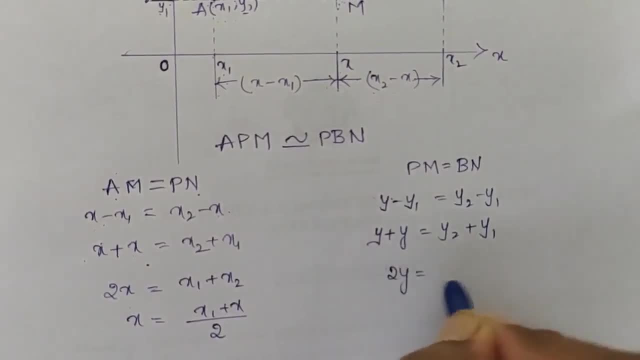 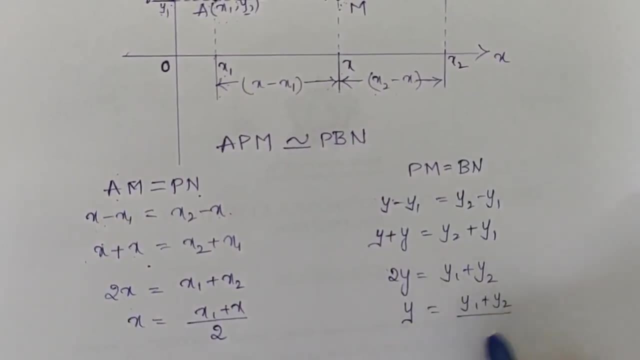 the y coordinate is 2y equals to y1 plus y2, and y coordinate will be y1 plus y2 upon 2. ok, We got the midpoint and we can represent it as p of x comma. y equals to x1 plus x2 upon 2. 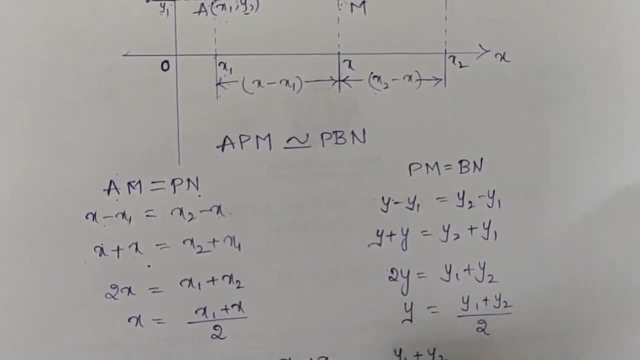 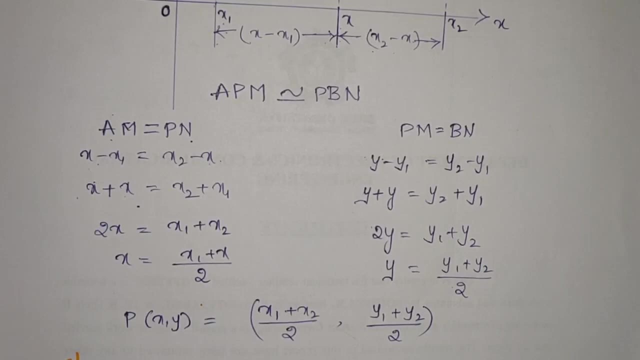 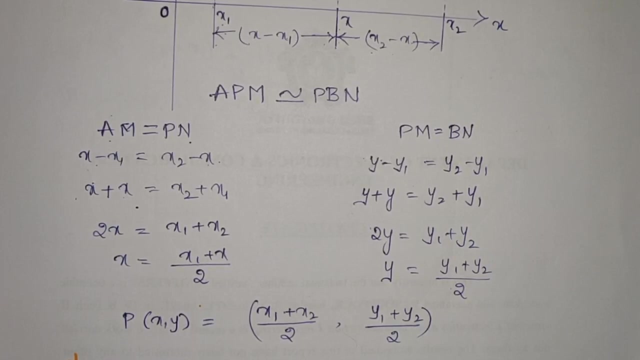 and y1 plus y2 upon 2 clear. Thank you for watching my video. Follow and subscribe our channel from innovative thoughts for more formula deductions and easy ways to solve problems, and reach out to us. You can also subscribe to my udemy profile for full length courses and link is given. in the description. Thank you,